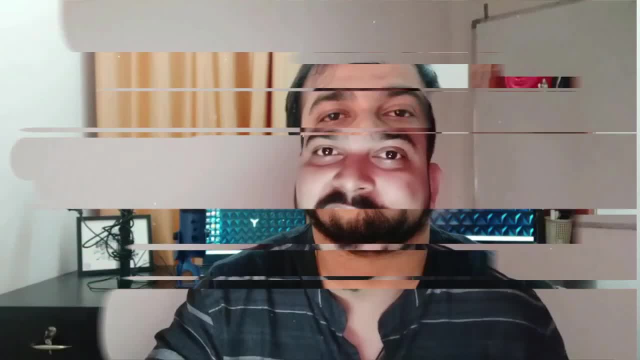 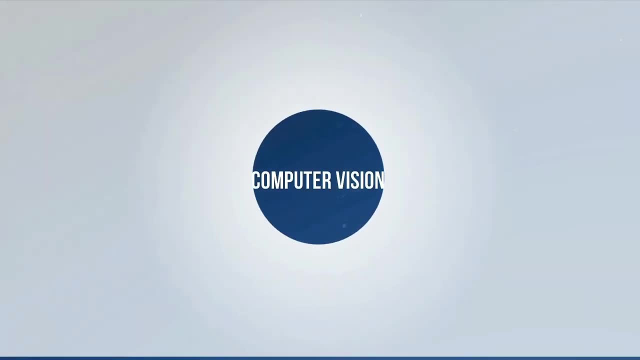 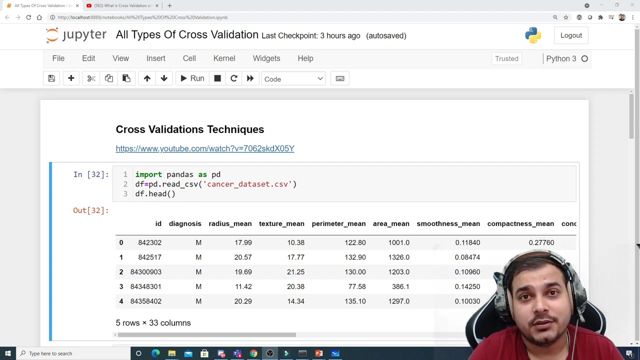 Hello all, my name is Krishnayak and welcome to my YouTube channel. So, guys, today, in this particular video, we are going to see all the different types of cross-validation. Now, cross-validation is very, very much important, guys. I had already uploaded one videos in. 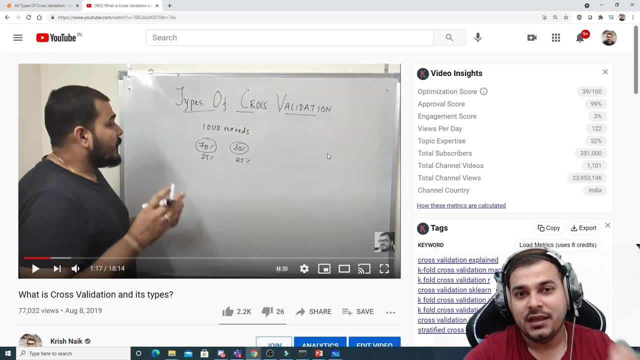 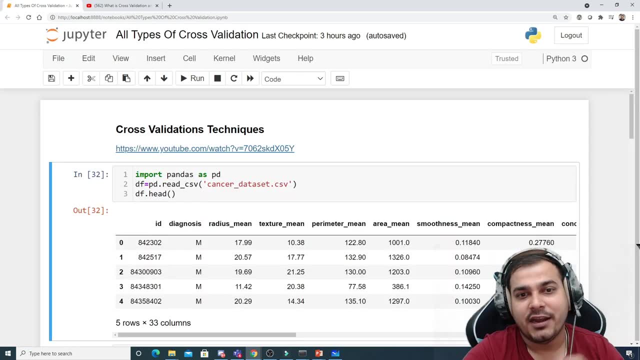 making you understand what are the different types of cross-validation, but here I just made you understand theoretically, So in this video we are going to understand how to do it practically and try to cover this. There are around four to five different techniques. 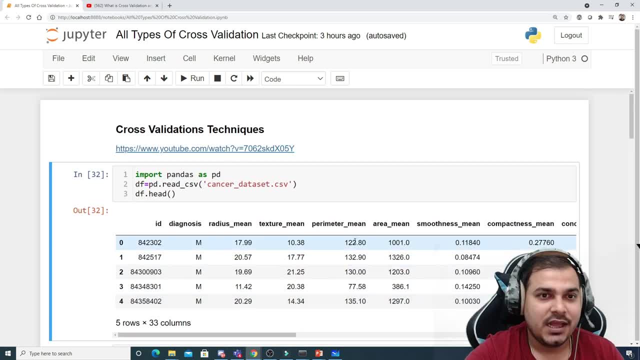 We'll try to see how we can actually do with Python programming language. And trust me, guys, when you are creating a machine learning project, in one of the most important life cycle is something called as hyperparameter tuning. In the hyperparameter tuning you 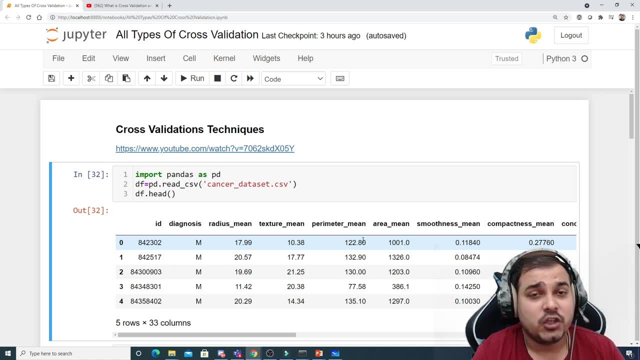 will definitely be using cross-validation techniques, So it is always good that you know what are the different types of cross-validation techniques and when you should use which one. So let's proceed In this particular example. what I'm going to do is that I'm going to 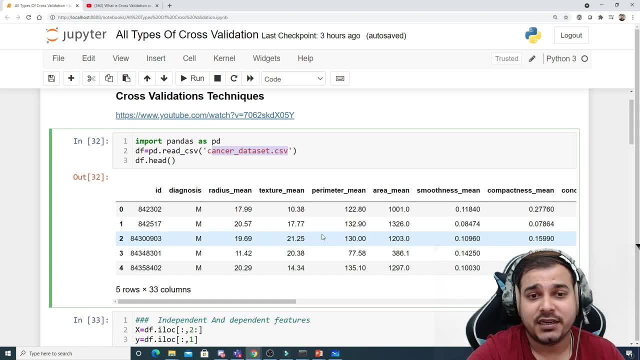 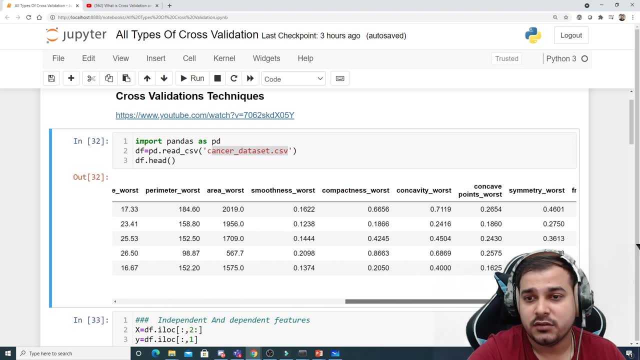 take a cancer data set. That basically means that in this particular data set you have data based on various features like this, like radius mean, texture mean, perimeter mean, area mean, smoothness mean. like this. Many features are there and you need to predict. 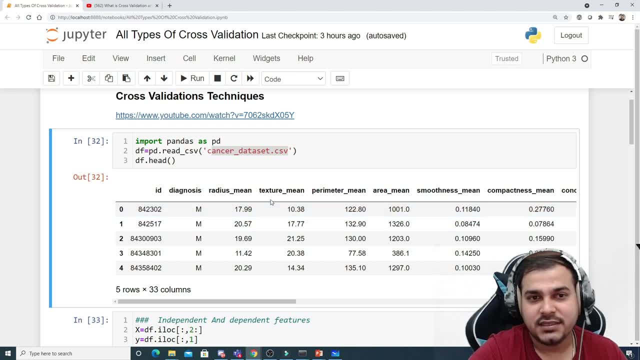 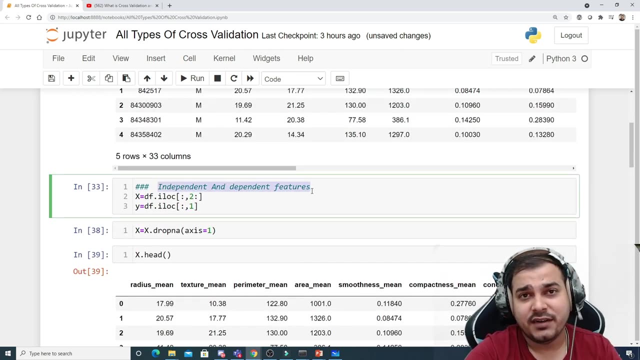 what type of cancer it is. There are two categories in this and that we need to predict. That is a simple, simple data set that we actually have. So initially we'll go and read this, We read this data set and this is my dfhead. The next step: I have to go and see my independent and dependent 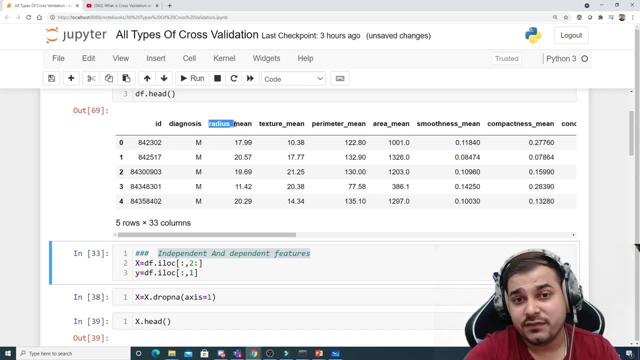 features. So obviously my dependent features- sorry, independent features- will be starting from this radius mean till the last feature And then this diagnosis is my dependent feature, this particular field, So from two to all the remaining columns I will be taking that as an independent feature and this ID column, you know, is not. 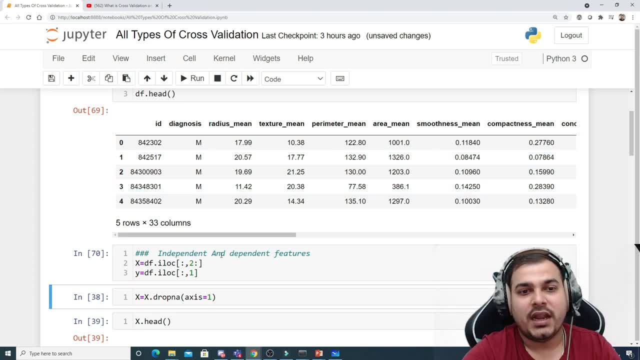 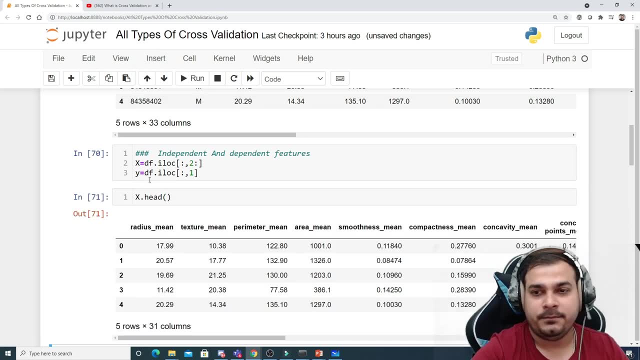 required because it is unique identifier. Okay, So I'll do that. So this is my independent and dependent features. So let me just go and check out my xhead. So here you'll be able to see all the features here. but one problem is there, guys. there is one more additional. 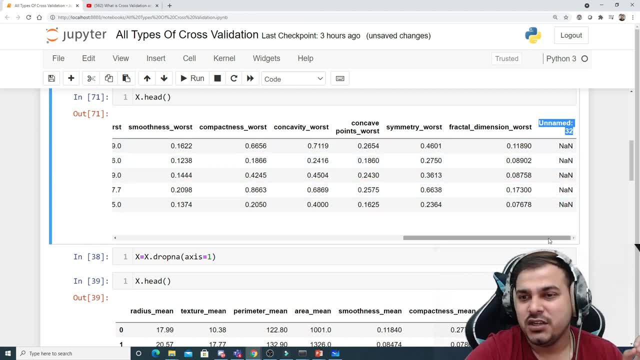 column, which is called as unnamed 32, which has all nan values. So it is better that we drop this particular column because it is of no use. So, in order to do that, I'm going to go ahead and create a new column. So I'm going to go. 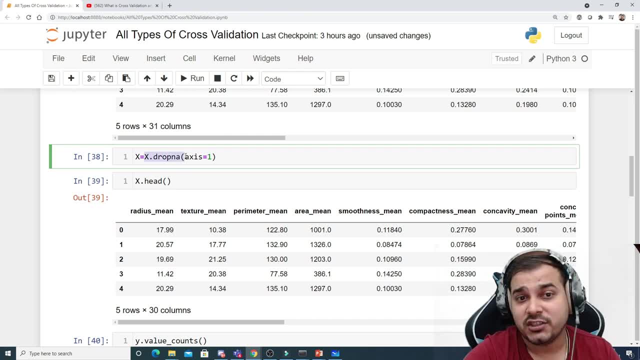 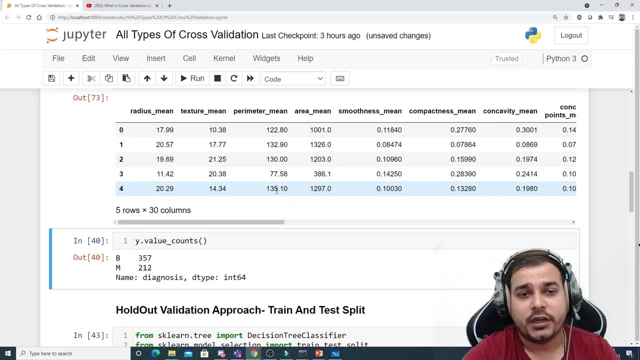 ahead and create a new column. So, in order to do this, what we are doing to do is that we are just going to write xdropna with axis equal to one, Perfect. Let's execute the next line of code. Now. we have this, our xhead. Now, in order to see whether the data set is: 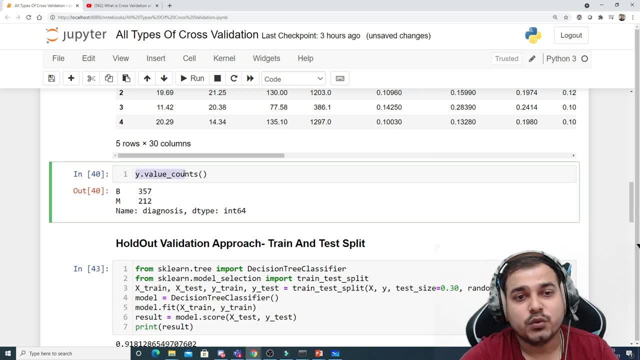 balanced or imbalanced or not. So what we do is that we can also use yvalue underscore counts. So here you'll be able to see: B category of cancer that is benign is somewhere around 357, and 212 is with respect to melanin. So right, So all this should be there, So let's. 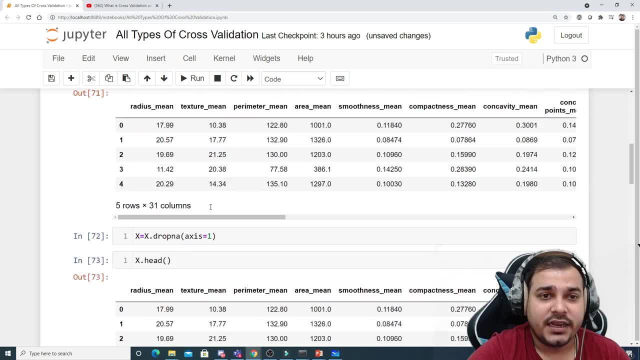 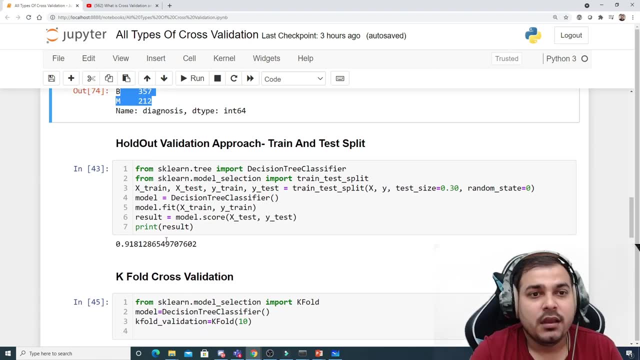 see what these two categories are. then, with respect to this, you have this, the data set I've actually taken from the Kaggle data set itself. Now let's go ahead with the different type of cross validation. The first technique that we usually use is called as holdout validation. 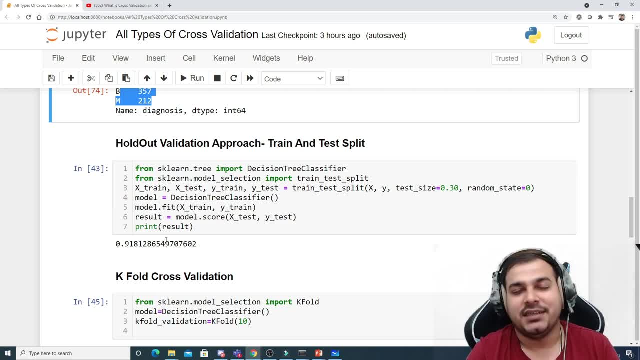 approach And in this we usually do a train test split. That's it. Most of the time you'll be doing train test split and that is nothing but holdout validation approach. This basically means that suppose if you have a data set, we try to do a train test split. 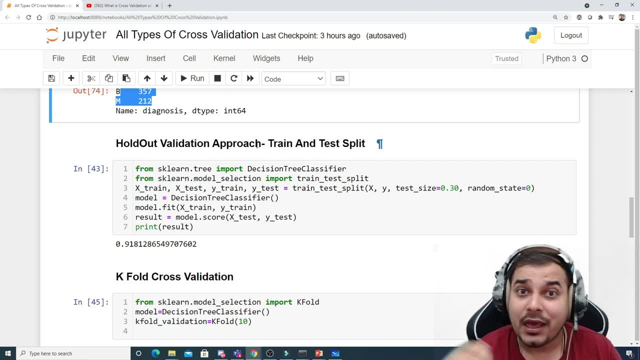 We train our model with the training data set and we validate our model with the help of test data set. So it's pretty much simple And I hope everybody's familiar with this particular technique, which we usually do because in most of the machine learning algorithms 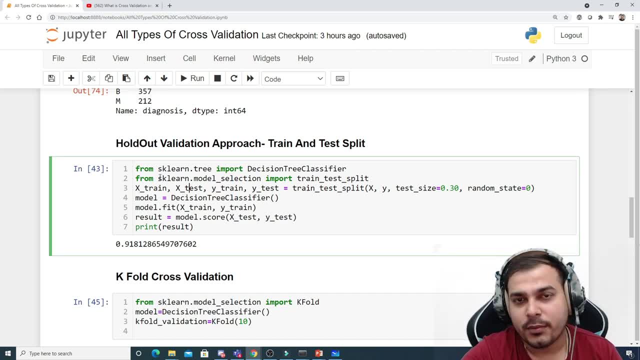 you usually go with this particular approach. So for this, uh, in this particular problem statement, I'm going to apply a decision tree classifier and then I'm also going to import this train test split and it is actually present in a scale on dot model selection, And then 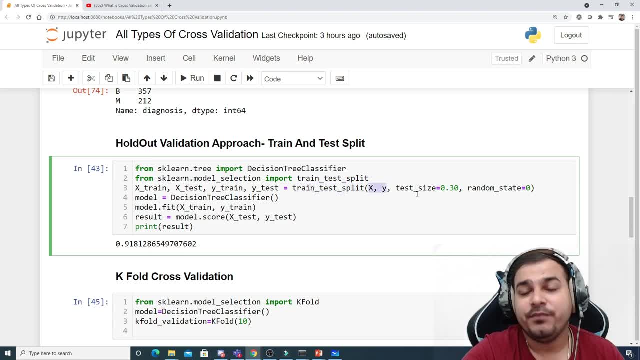 after using train test split, I just have to give my independent dependent feature My test size, which is nothing but 30%, and the random state is equal to zero. here I'm just initializing decision tree classifier, guys. Remember after this you can also perform. 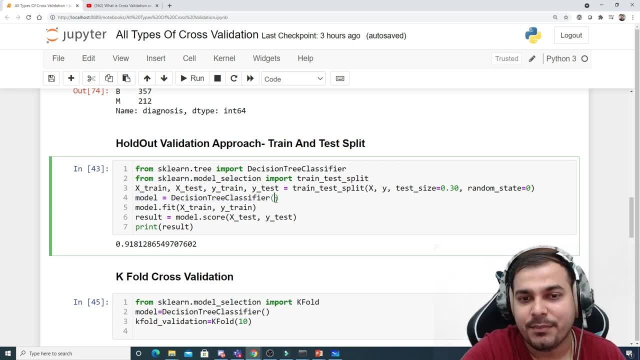 hyperparameter tuning. It is not only because here I've not provided any parameters. All the parameters are default. If you want to provide your own parameters, provide a go and go ahead and do the hyperparameter tuning. But just to show an example of different types. 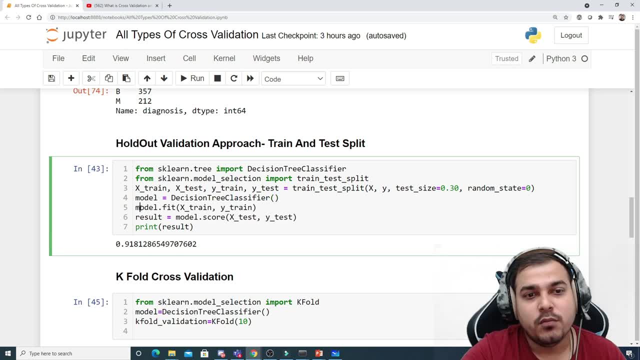 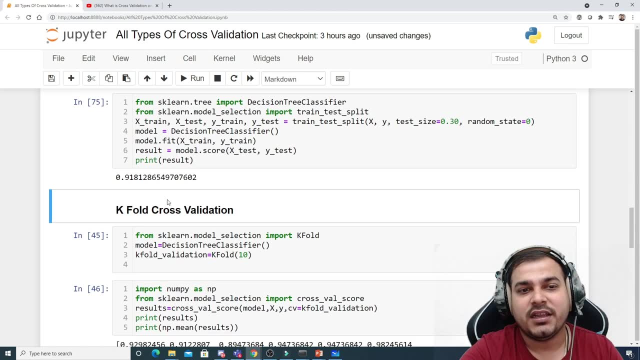 of cross validation, I'm using this particular approach. Then we do model dot fit on extra invited And then, finally, we find out the model dot scroll on X test, Y test. So once I execute this particular result here, you'll be able to see that I'm having 91%. So, guys, let's. 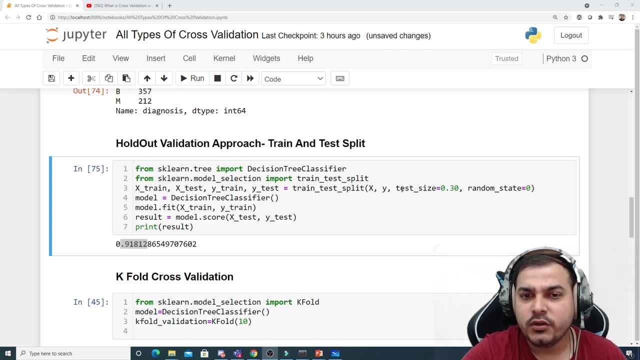 understand the disadvantages of this. Now here you'll be able to see that we are just doing us a single type of train test split And that that train test split is defined from this random state value, because it will be just randomly selected right, 70% will. 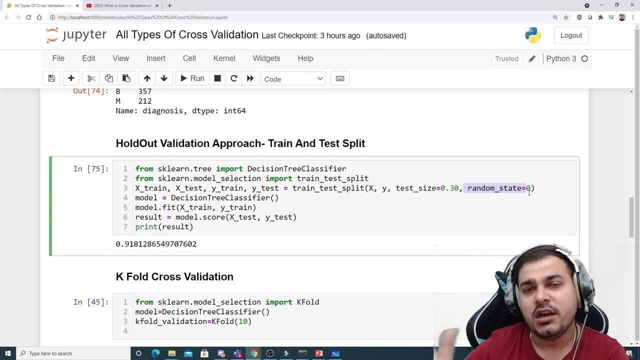 be selected in our training data set. 30% will be selected in our test data set Right now as I go on changing the random state. so suppose if I go and change it now you can see that the percentage accuracy is 92%. Now suppose if I make the random state, 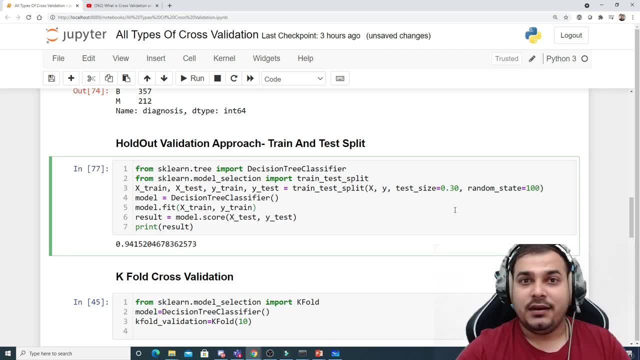 as a hundred. again it can become 94%. So we don't know like how randomly the um, you know, the train test split may happen and we may get different, different accuracy. So this may actually lead it to overfitting. Also, it may also lead it to underfitting. 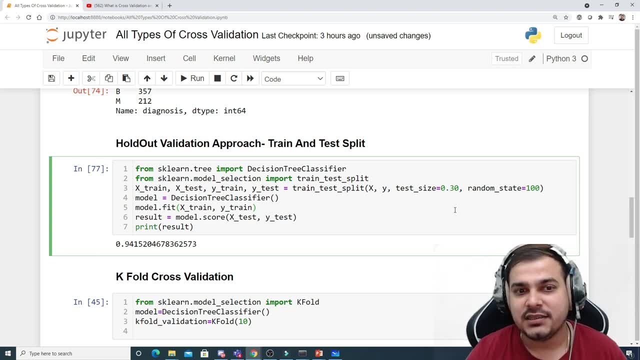 also because we don't know, based on the random state, how we are splitting the data set. We are getting the accuracy Now in order to overfitting. we are splitting the data set. We are getting the accuracy Now in order to overfitting. we are splitting the data set. Now, in order to overfitting, we are splitting the data set. Now, in order to overfitting, we are splitting the data set. So, in order to overcome this, what we do is that we go with the second type, which is: 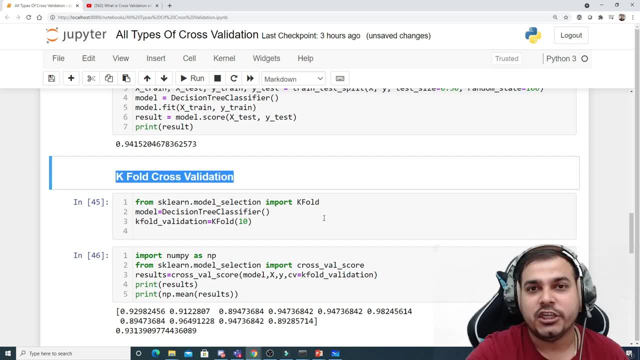 called us K-fold cross validation. Now, in K-fold cross validation, we can make around 10 splits, 20 splits, based on our uh, you know. and again, how to select that particular split value. I will, I'll talk about it also. Now, in K-fold cross validation, suppose, if 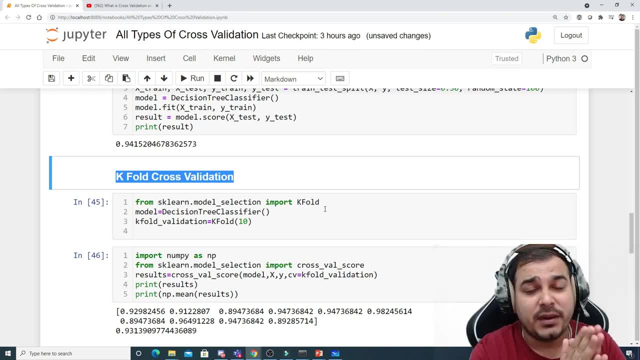 I say that I'm going to do 10 splits, so 10 different splits of train and test data will be taken. for all the different splits We'll try to apply a machine learning model and then we'll try to see what will occur. 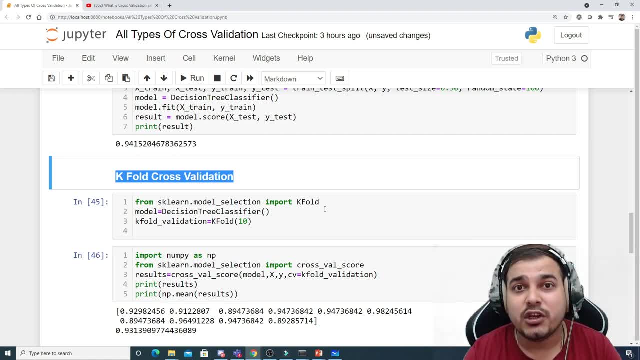 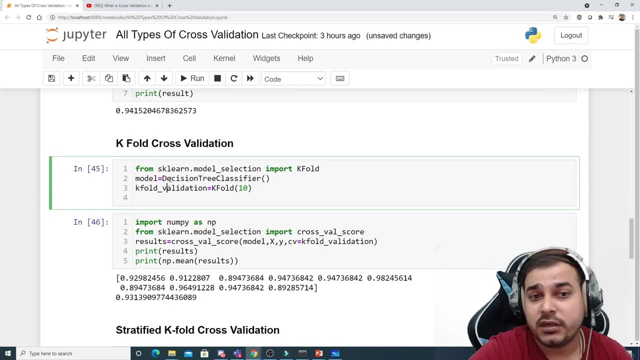 accuracy we are getting. finally, the average mean of the accuracy is actually taken and told to the stakeholder right. this is how you have to actually mention. now, in order to perform k fold, k fold, cross validation, we just have to use sklearnmodel selection: import k fold. then i am going to 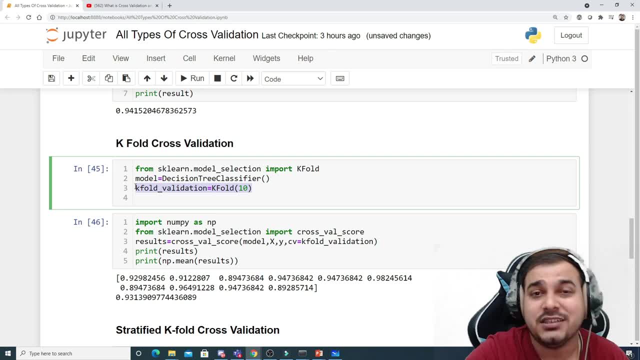 initialize decision tree classifier. now here you see this how i am initializing the object. so i have created k fold underscore validation and here i have to use k fold as 10. 10 basically suggest that i have to do 10 different splits. now what is this? 10 different splits, just let me. 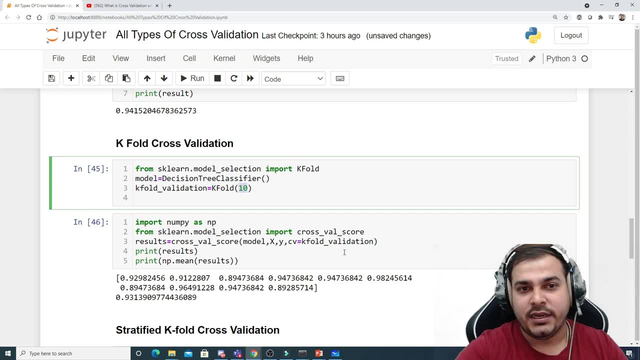 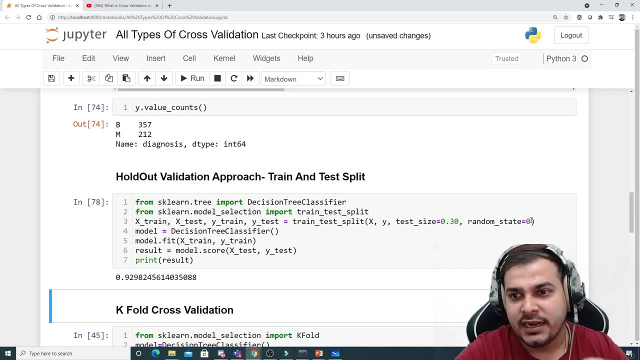 make you understand. suppose i have a data set in the first split. consider that it is going to select a random state as zero and it is going to do some kind of train test split, right? then again with the the second split, maybe with respect to another random state, right? so like this multiple. 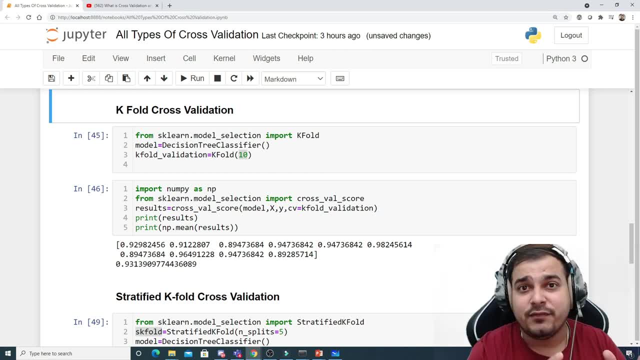 splits will be taken and with respect to each and every split that have that we have done and got the training and the test data set, we are going to apply it for our machine learning model and get a separate accuracy. so all the 10, if i am doing 10 splits, i am going to get 10 different. 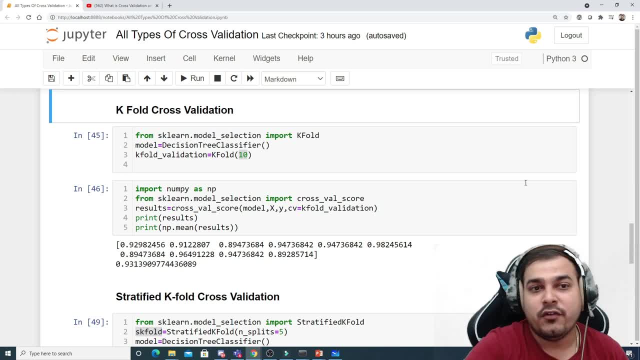 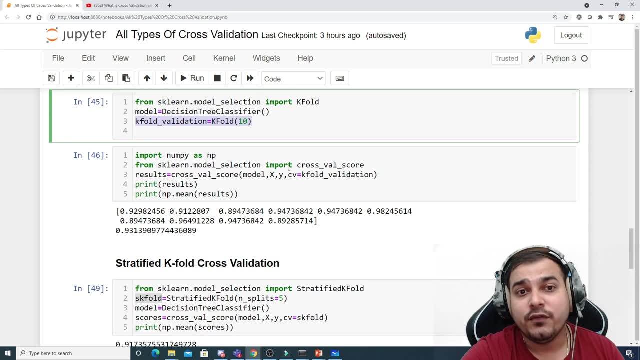 accuracy. okay, so this is the importance of k fold cross validation. now here. by doing this, we will be able to get the 10 different splits of trend test data and then, in order to verify and pass it to our model and see the accuracy, what we do is that we use something called as cross val score. 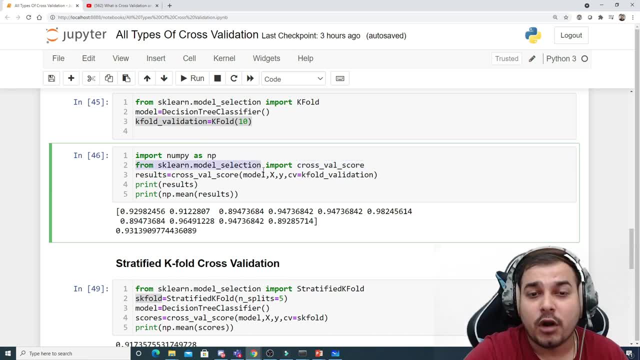 so for this we will be using from sklearnmodel selection import cross val score. in the cross val score we provide our model and we will be able to get the 10 different splits of trend test data model. our x, y and cv is equal to k fold underscore validation. this cv is nothing but cross validation. 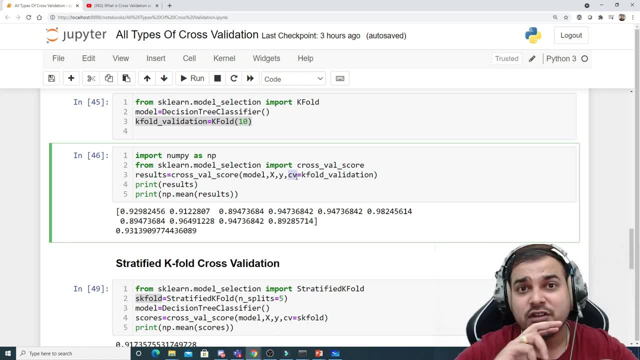 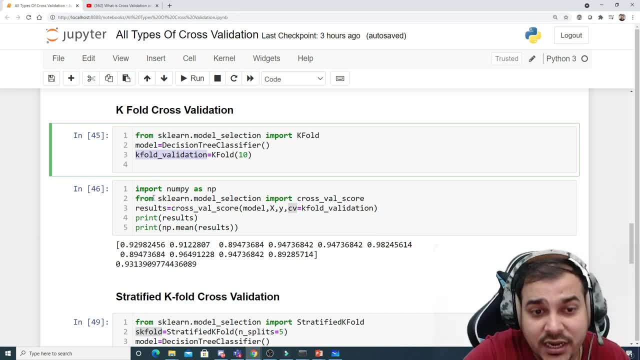 okay, cross validation. that basically means how many different types of trend test split are there here. we know that in our k fold underscore validation, it has 10 different types of train and test split, so the results that we are actually going to get will be a list of 10 different. 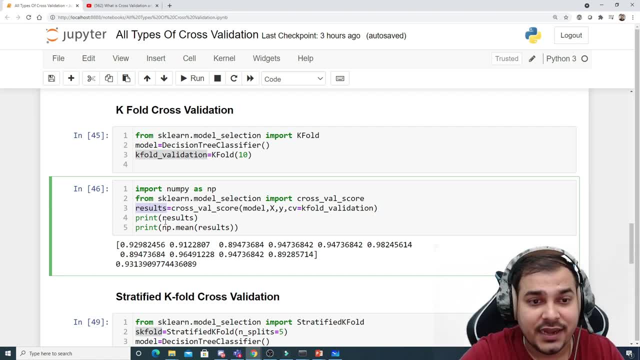 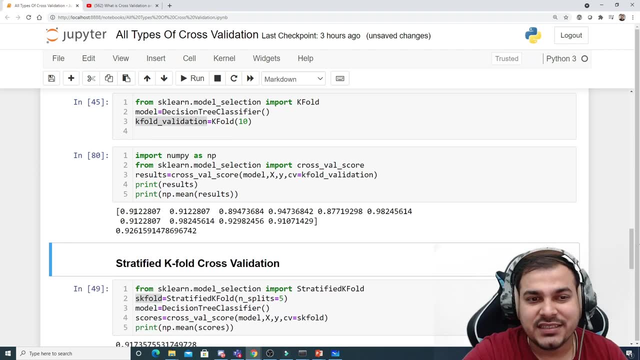 accuracy values. okay, so if i go and execute this, and here in the last line, what i'm doing, i'm doing is i'm going to get the mean of that particular result. now, here it is. now here you can see that 10 different experiments. let me count one, two, three, four, five, six, seven, eight, nine, ten, so 10. 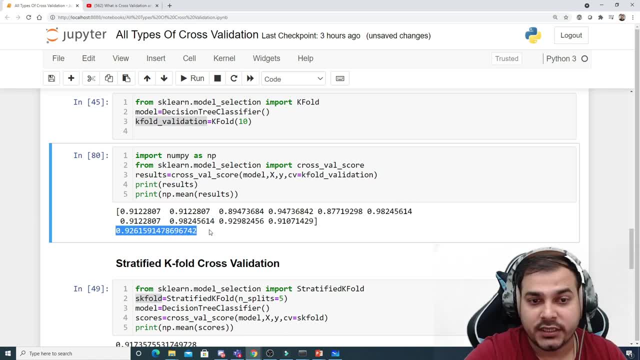 different experiments are there and when we did npmin, i'm getting 92 percentage accuracy right now. how? how to decide that, whether i have to go with 10 splits and all again. it is a hyperparameter, tuning parameter, but understand that. how do you have to tell this particular information to your 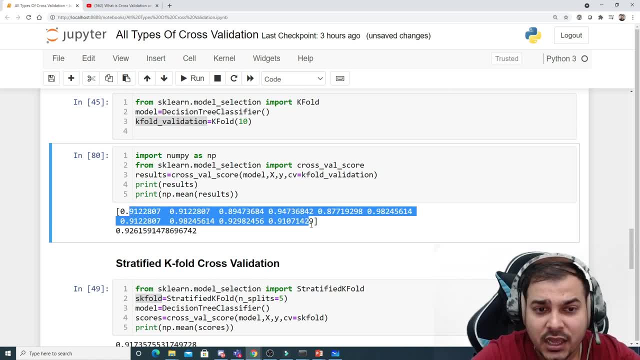 client. okay, now, from all this particular accuracy guys, you will be able to see that you are getting the least accuracy as 87, and the maximum accuracy that you are able to get is somewhere around 98 percent. so just to the stakeholder, when you are defining this kind of model, and most of the time 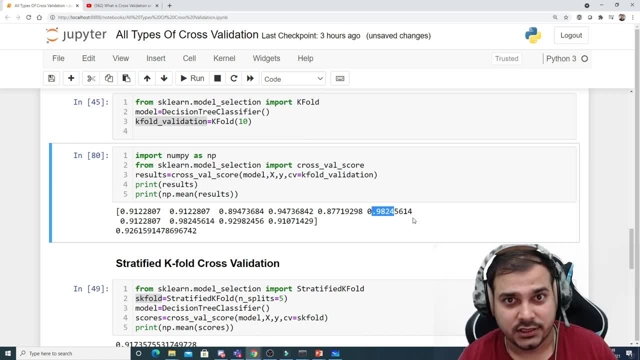 we usually go with this particular technique unless and until your data set is not balanced okay. so if i was getting this kind of accuracy, i used to say my stakeholder that, yes, the maximum accuracy that i have actually got is 98 and the least accuracy that i have actually got is 98. 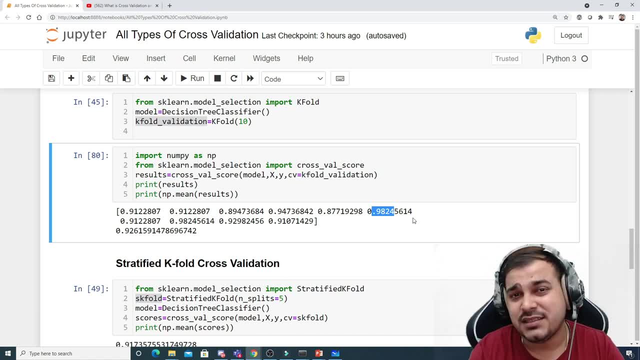 actually got is somewhere around 87. so by this, the mean accuracy that i would like to say is somewhere around 92. okay, so this range, when you say right, and if this range is quite huge, again we have to do some kind of hyper parameter tuning. if the range is very, very small, then no need of doing. 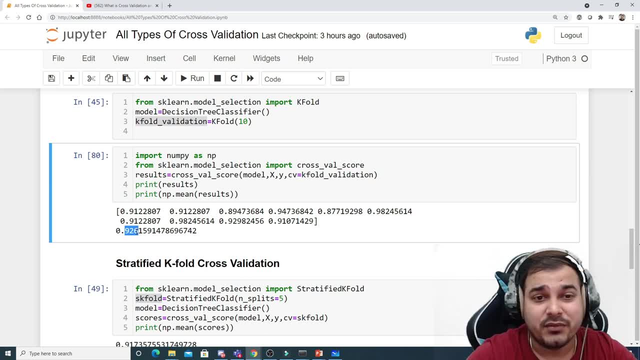 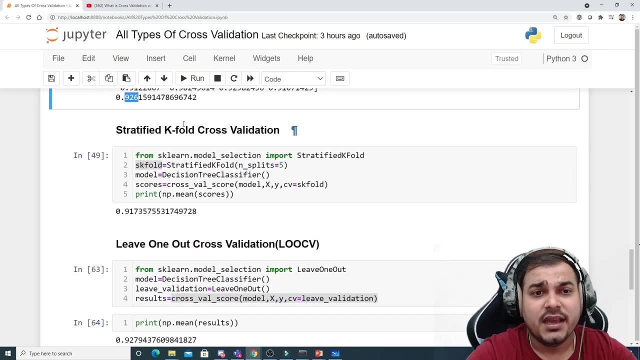 the hyper parameter tuning and your managers will be pretty much happy with this specific result. so the second type that we have discussed is k-fold cross validation. now let's go with the next type: stratified k-fold cross validation. now, remember guys in stratified k-fold correlation. 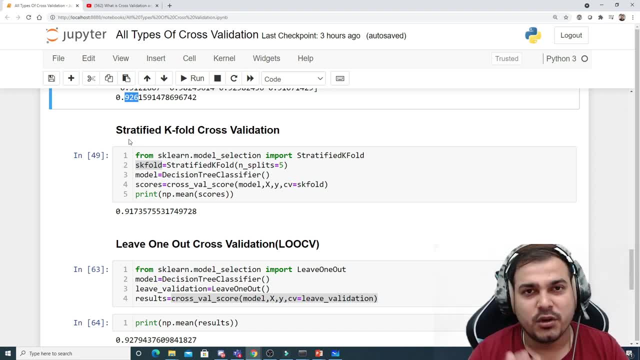 what happens if your data set is imbalanced? suppose if you you have uh, the data set in which your one category count is somewhere around 900 and the second category- suppose if i'm considering a binary classification problem- and the second category count is somewhere 100. so this ratio is: 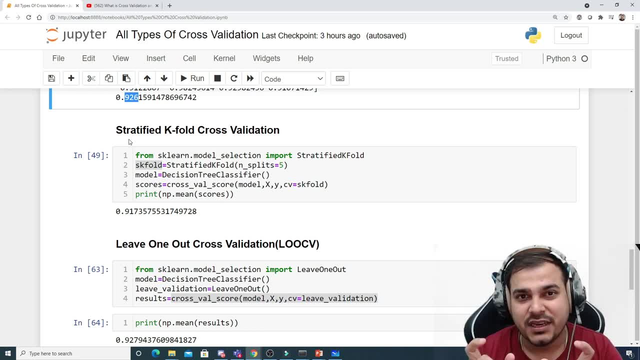 nothing but 9 is to 1. right now, when you have the specific ratio and if i try to do a train test split of cro uh, this k-fold split, you know, correct proportion of elements will not be picked up with respect to both the categories. it may be a situation that all, all the categories that are selected will be from. 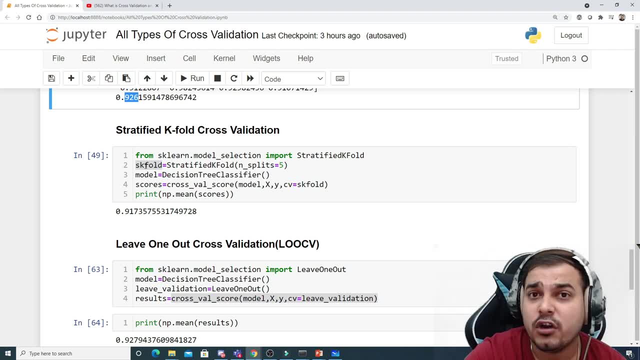 one category only, right. so stratified k-fold cross validation makes sure that if we have an imbalanced data set, if you are doing a train test split, it will make sure that our independent with respect to our dependent features- both the categories- proportion will be taken in an approximate equal amount. okay, now suppose if i take an example, 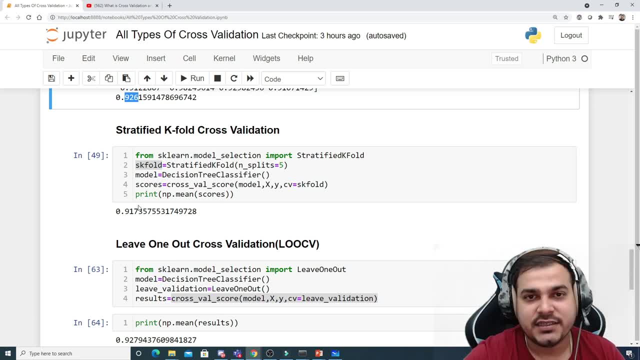 suppose i have 700, uh 700 data sets. uh, probably with yes, 300 data set, probably with no. now if i try to apply k-fold cross validation, suppose my 70 percentage of the information is there- 70 percent i'm giving in my train test split. so what it will do, it will try to take around 500. probably- i'll not say 500, at least 400 from one category and 300 from the other category. it will approximate the number of categories that is is going to take from both the classes. okay, so stratified k-fold cross validation will be definitely used in an imbalanced data set. 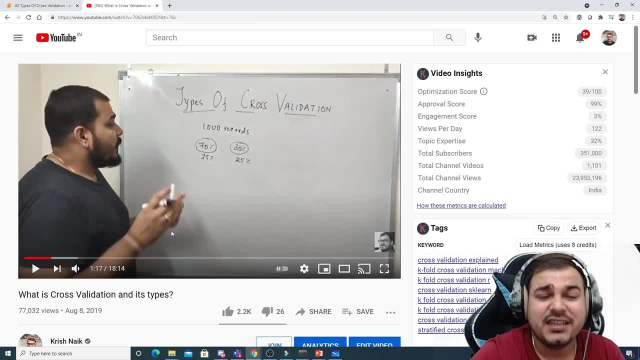 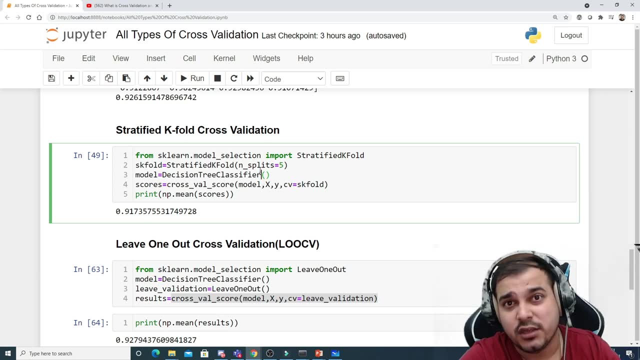 pretty much simple. and again, guys, all these things has been explained already in this particular video. i've explained detailly, you don't have to worry about it. this someone had requested me to put the practical video also, so i'm actually creating this particular video. so from escalonmodel. 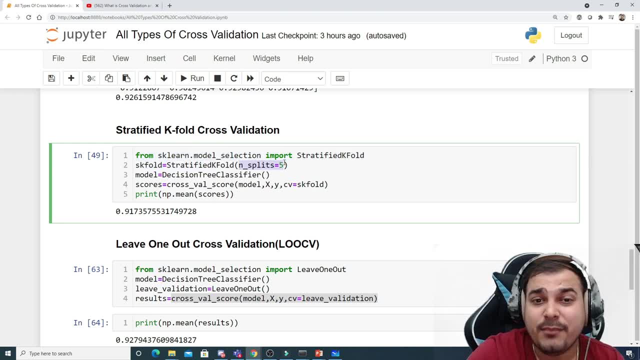 selection imports stratified k-fold, and in this particular k-fold i'm doing five splits. now if you go and see this particular splits and if you see the count of the data set of the data with respect to the categories, it will be approximately equal. then again, i'm using 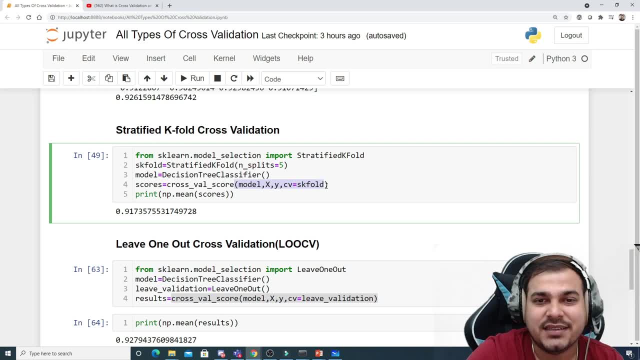 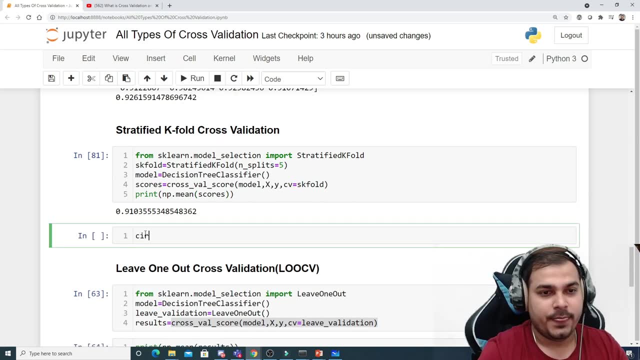 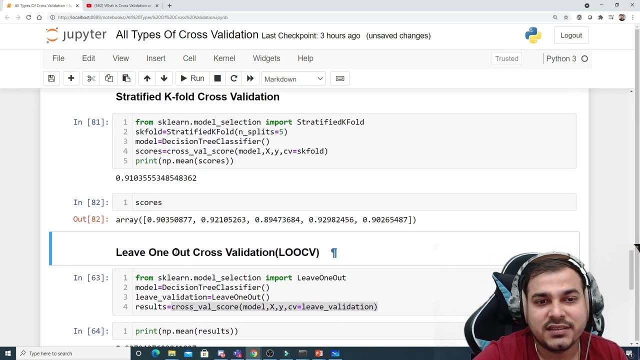 crossval score and i'm giving model x, y, c, v, s, k a fold and i'm just trying to see this particular score. now, if i also want to see my scores, you'll be able to see this and again. guys, all the values will be varying. you need to know when to use what. so here you can see 90, 92, 89, 92, 90 and the average. 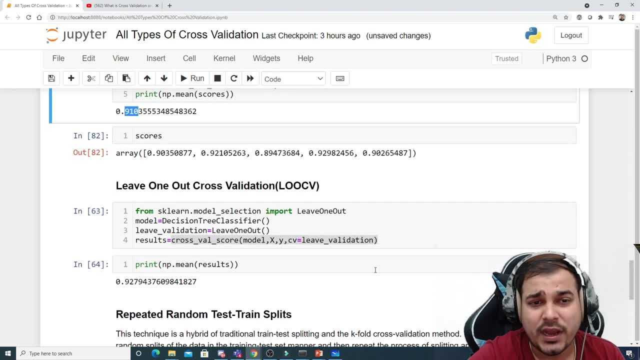 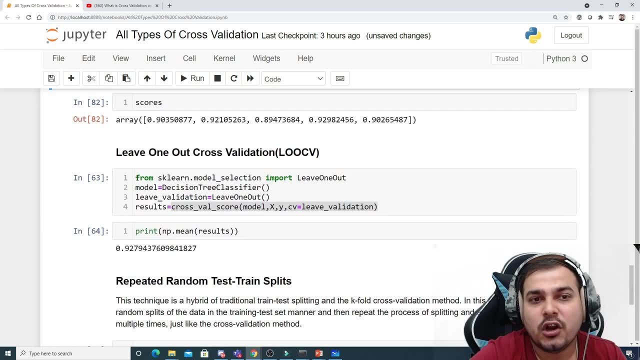 accuracy that you're seeing is 91.. now, coming to the last one, and always remember, when do you use stratified k-fold cross validation? when you have an imbalanced data set, then, uh, you have something called as leave one out cross validation in this. what you do, it is very, very simple from the entire. 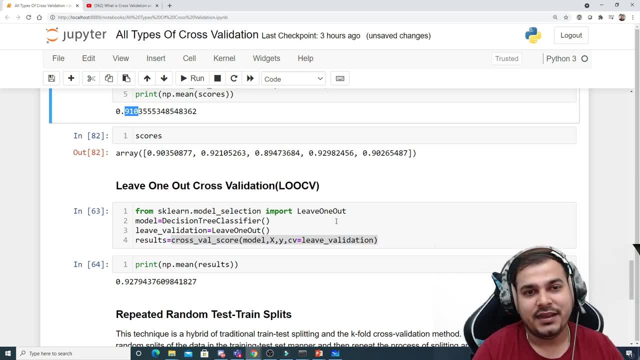 data set. you take only one data. you take it somewhere, right, this is leave out. leave one out cross validation. there is also like leave p out cross validation. p basically means i'll tell you, okay, so in leave one out cross validation, what you do from the entire data set you take. 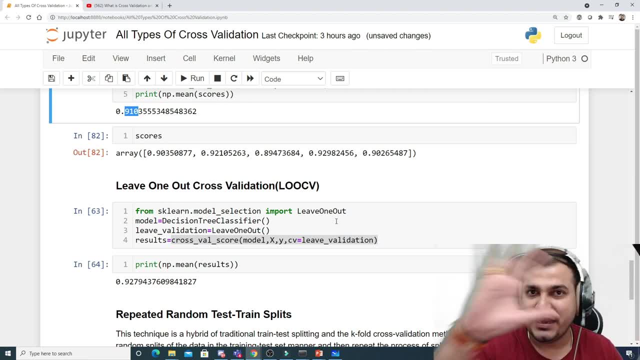 you pick up one data randomly as your touch data and remaining all your values are you're going to will be your training data. like this, you do it for every sample. suppose you are going to take, suppose if i, if i say that i'm going to perform this, leave one out on a data set based on the. 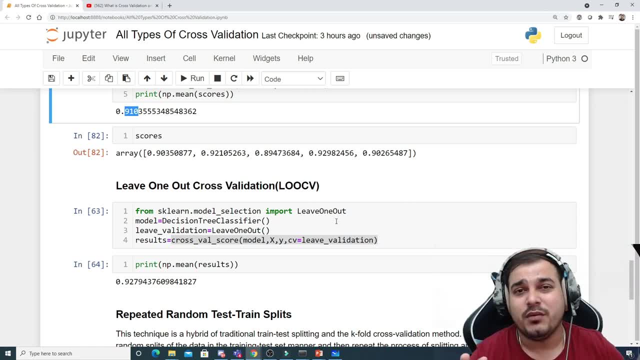 number of records. every time i'll pick up one record. all the remaining record will be actually my training data set. then i may go and pick up my second record as my test and remaining all records will be my training data set. so like this i'll be continuing doing all the operations and over here. 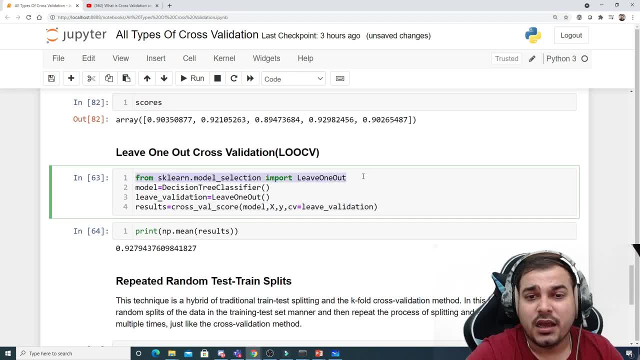 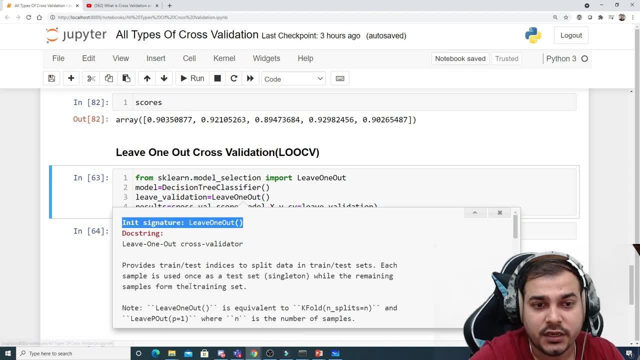 in order to perform this. here you'll be able to see from a skill learned model: uh selection. i'm going to leave one out if i go and see this particular parameter. guys, here you'll be able to see all the information right. uh, here it is saying they leave one out. cross validator. 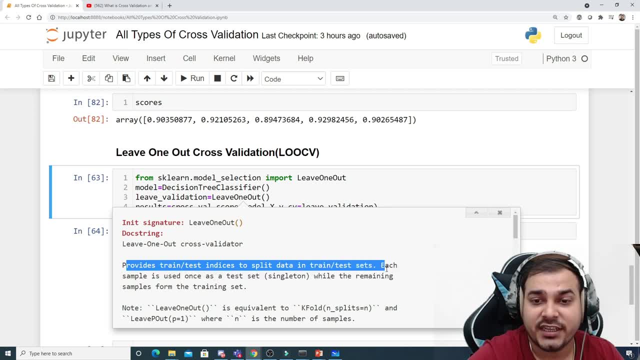 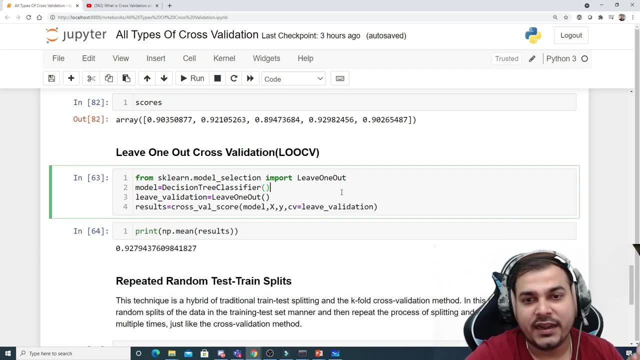 provides train test indices. to split the data set into train test split. each sample is used as once as a test data, while the remaining samples from the training set. now, if i try to execute this okay, it will take some time. this will be the slowest because based on the number of records. 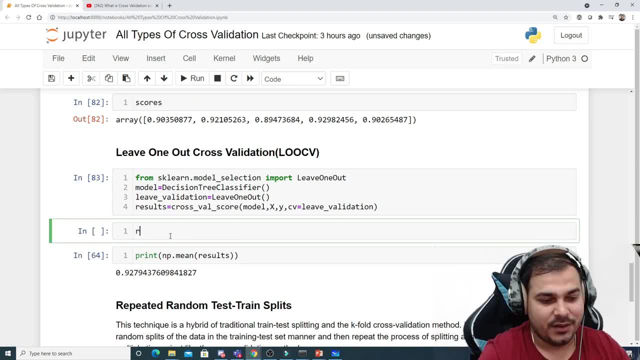 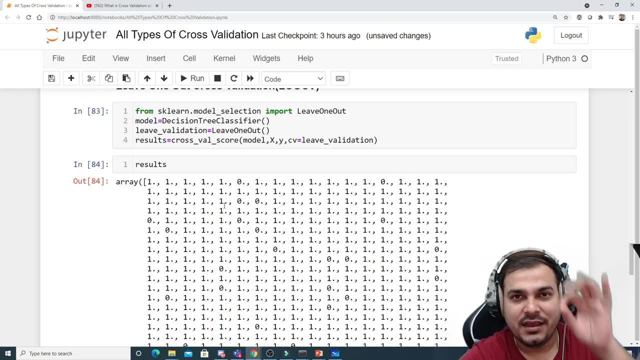 right now. if i go and check out my results, you'll be able to see that how many data sets i'll be having. this many number of values, so this many number of different, different samples they have taken by selecting one as a training data set, test data set and remaining all as a training data set. 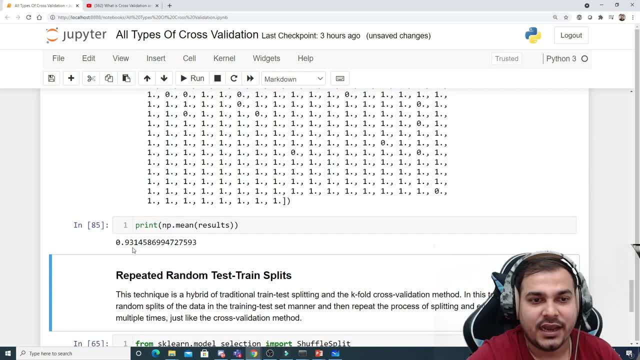 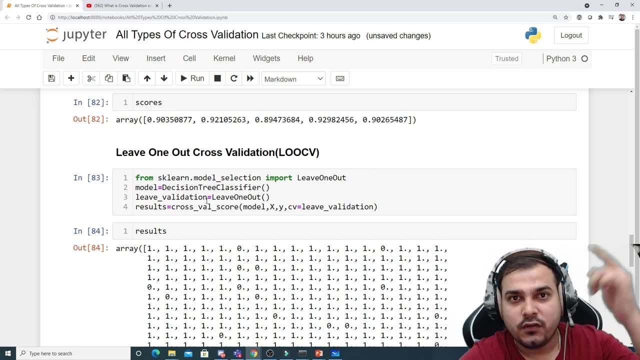 so, finally, if i use np dot mean, then here you'll be able to see 93. okay, now, this is perfect, guys. there is also something called as leave p out cross validation. instead of one, you can also specify values like: i want three, four, five. that basically means from the entire data. 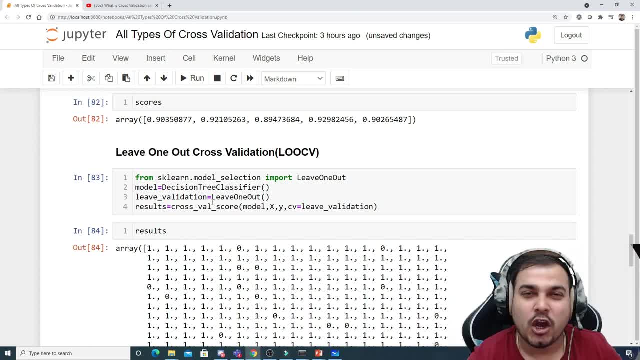 set. in every iteration we take our three data set remaining all over by training data set, and this will be a test. then again we select another three, then we go like this right. so again. uh, i'd suggest that this is usually a cubism process. it is hardly done. uh, you should not try to do this. 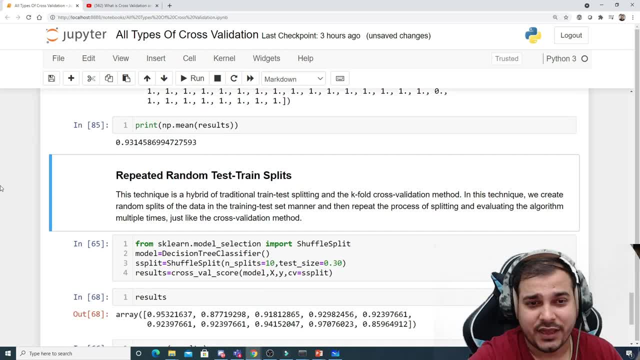 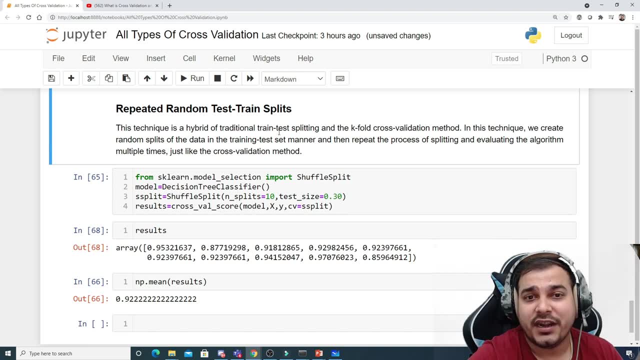 because in a real world scenario you have millions of data set, it will take a lot of time. now this is another one, uh, which is called as repeated random train test split. now, this technique is a hybrid of traditional train test split and and the k-fold cross validation. 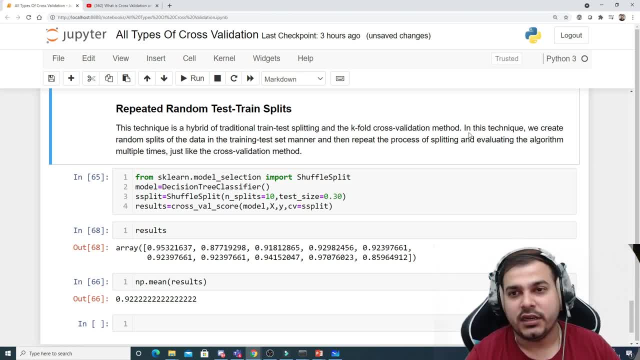 method. so train, test splitting also and k-fold. it is a combination of that. in this technique we create random splits of the data and training, test, set mana and then repeat the process of splitting and evaluating the algorithm multiple times, just like cross validation method. pretty much simple.